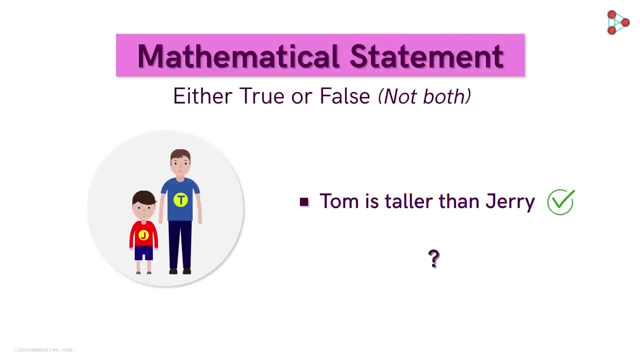 Yes, this is a mathematical statement. Why do I say so? As the heights of Tom and Jerry can be measured, we can always verify the statement. It will either be true or false. So this is a mathematical statement. Now let's look at a few more statements. 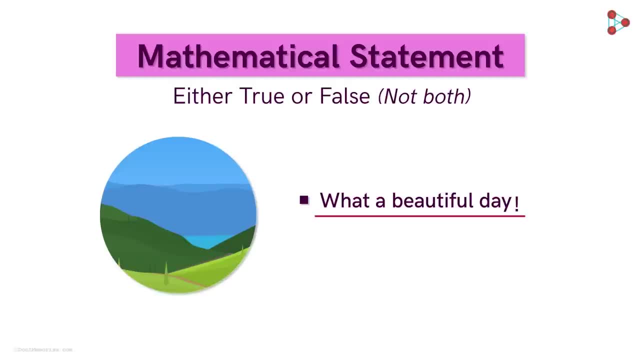 Here's the first one: What a beautiful day. Is this a mathematical statement? It's not, Because an exclamation can never be a mathematical statement, So the statements like Wow and The food was amazing are also not mathematical statements. Here's another one. 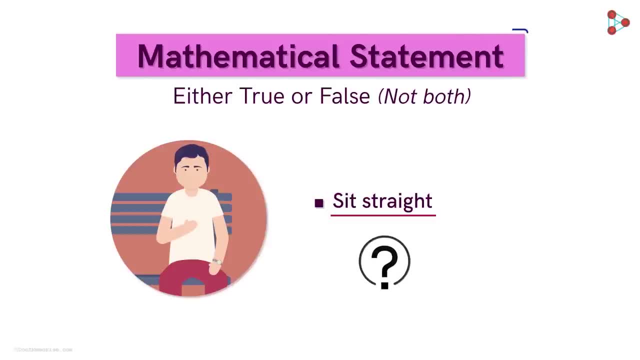 Sit straight, Mathematical statement or not. Notice that this is an order, And an order can never be a mathematical statement. So statements like Open the door and raise your hand are also not mathematical statements. Okay, next, All squares are rectangles. What do you think? 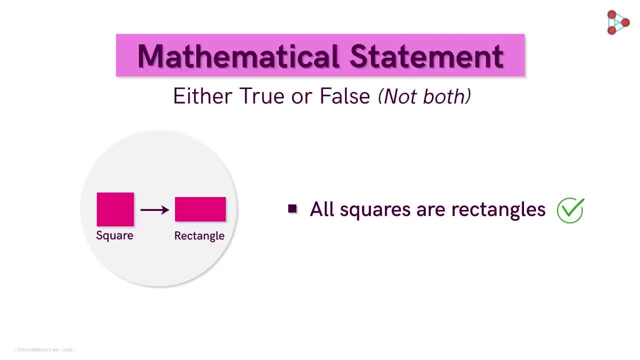 Yes, it's a mathematical statement, Because we can definitely say that it's true. Next, What is your name? This is a question, And a question can never be a mathematical statement. What about these two statements? Here she could mean any girl and here could be any place. 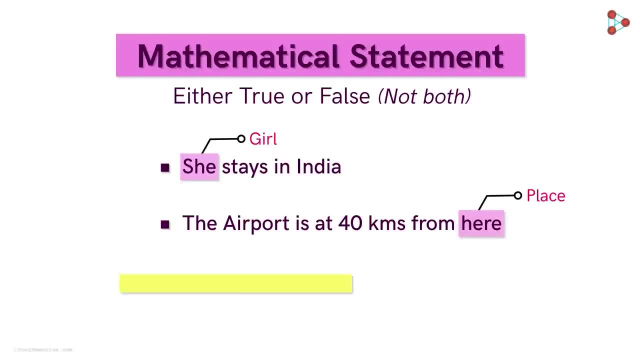 She, and here are pronouns, and statements involving pronouns cannot be considered as mathematical statements. Are you ready to try out a few more examples? Okay, here we go. Consider this statement: The sides of all the quadrilaterals are equal. Is this a mathematical statement? 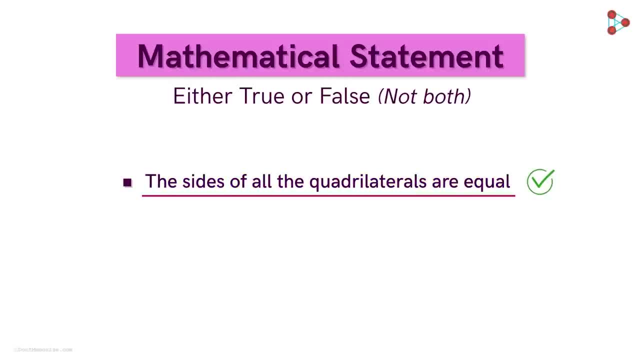 Yes, it is, Because we definitely know that it's a false statement. Remember, it could either be true or false. It doesn't only have to be true. Okay, now for the final two examples. Here they are. Is this one a mathematical statement? 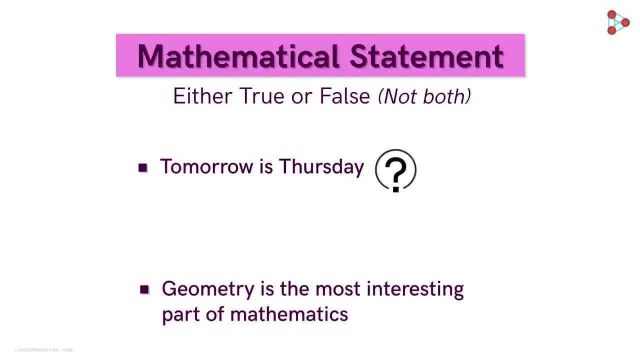 We should know that statements involving variable time, such as today, tomorrow or yesterday, are not considered to be mathematical statements. Why This example? for instance, will be true only on Wednesday and not on any other day. So it may be true or false.